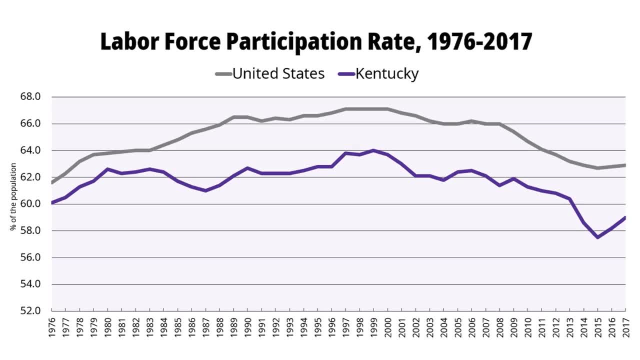 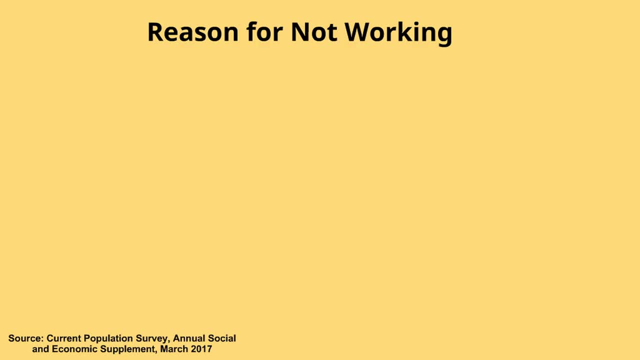 Kentucky's low labor force participation rate is not a new trend. Kentucky has historically had a lower labor force participation rate than the United States as a whole. There are many reasons why an individual would choose not to participate in the labor force. For those who did not work last year, almost half were retired, Others were going to school. 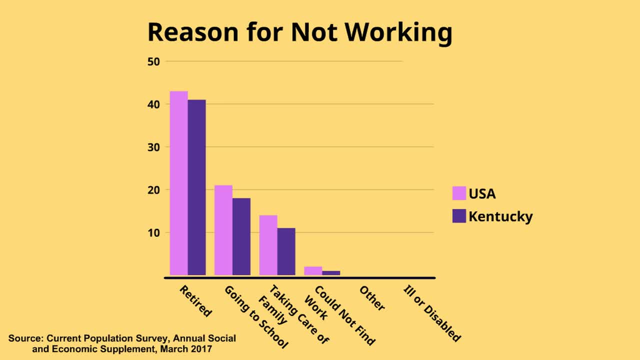 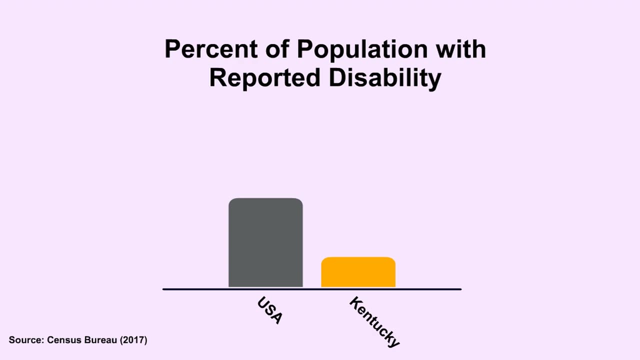 taking care of family or were unable to find a job. Less than 2 percent of individuals did not work last year for unspecified reasons. Compared to the United States, Kentucky has an exceptionally high percentage of labor force participation rates. The percentage of the population reporting a disability in Kentucky is five points higher. 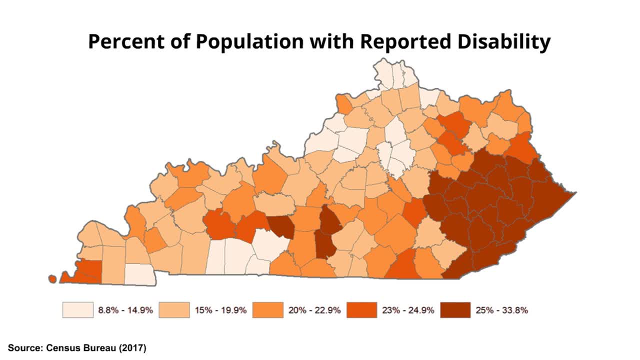 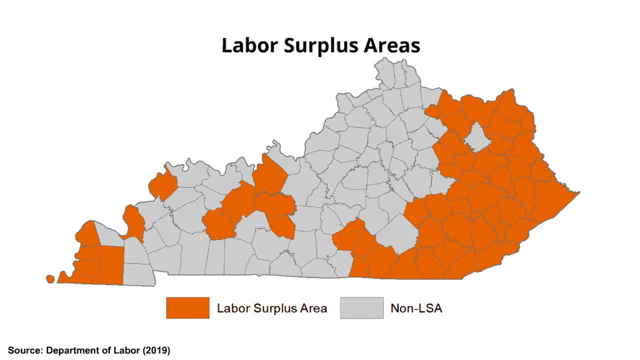 than the nation, and in the eastern part of the state, many counties have over a quarter of their population reporting a disability. These areas also tend to suffer from a shortage of jobs, making it difficult to find work even for those who don't require special accommodations. There are 52 counties in Kentucky federally designated as labor surplus areas because there are persistent labor shortage areas. Kentucky has a low labor force participation rate in the state of Kentucky and there are significantly more available workers than jobs. For many people in Kentucky non-participation in the labor force is not always a choice. 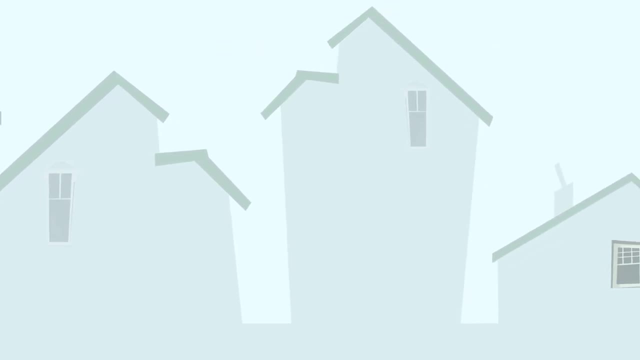 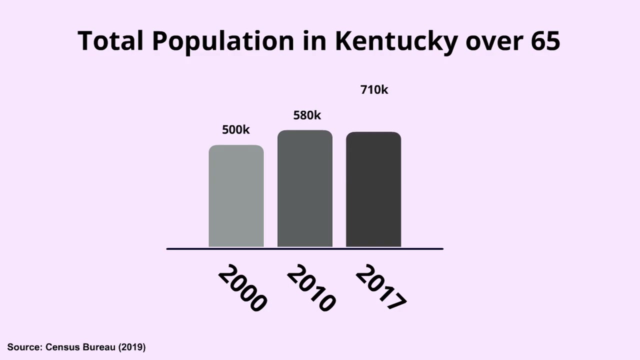 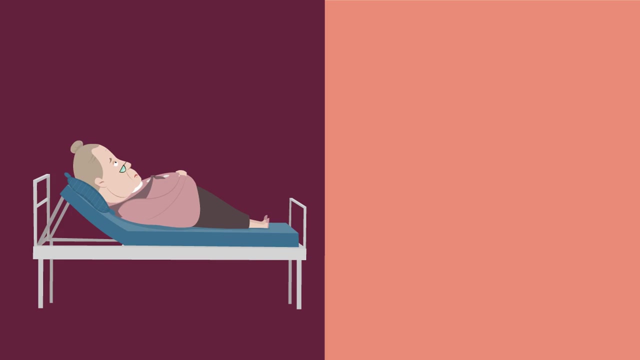 but rather a consequence of systematic economic problems in their communities. Another factor driving both the increase of disabled Kentuckians and low labor force participation is the aging of the population. Older people are more likely to drop out of the labor force because illness prevents them from working or because they choose to retire Current. 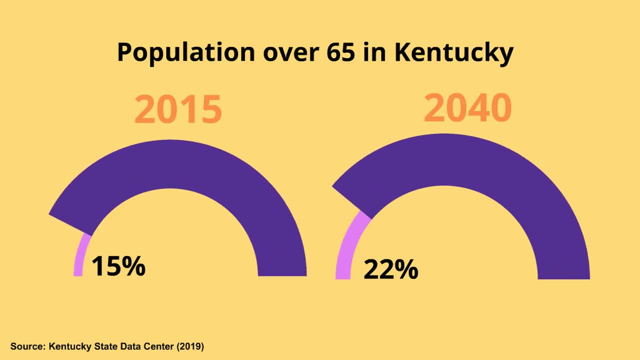 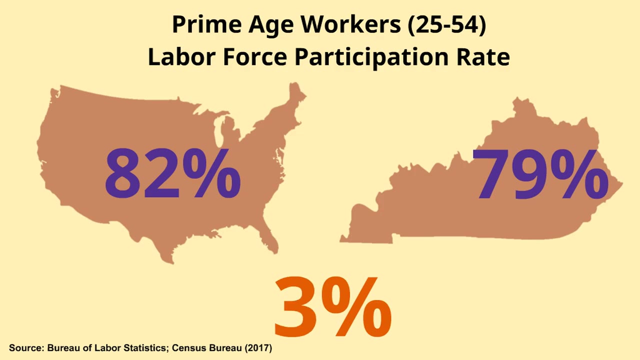 population projections show the proportion of the labor force in the state of Kentucky is more likely to drop out of the labor force because illness prevents them from working or because they choose to retire. Kentucky's labor force participation rate jumps 20 points and is closer to the national. 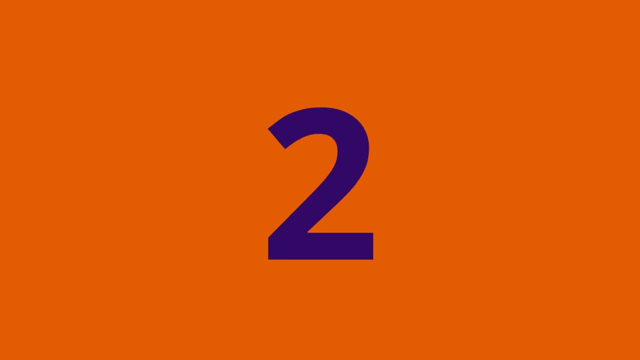 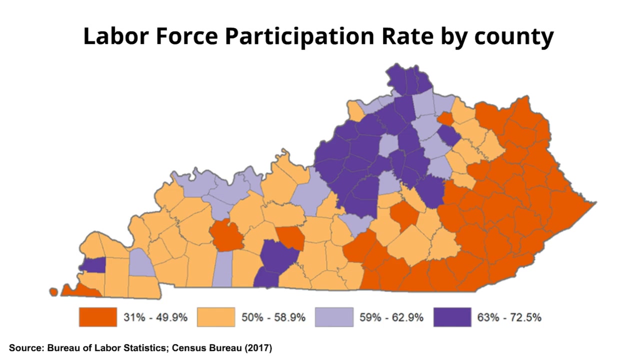 average. Two primary forces are driving the low labor force participation rate in Kentucky. One: Kentucky's low labor force participation rate is a consequence of an increase of work force participation in Kentucky than in the state öll of its urban-rural divide. 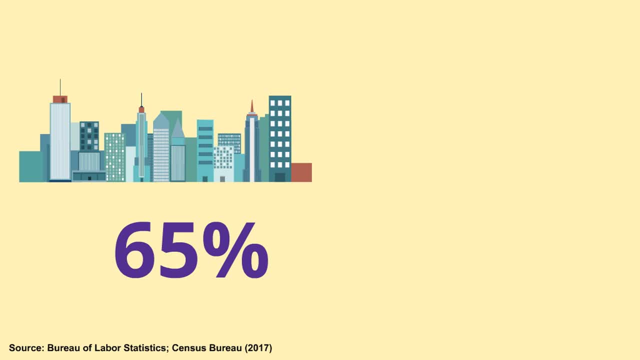 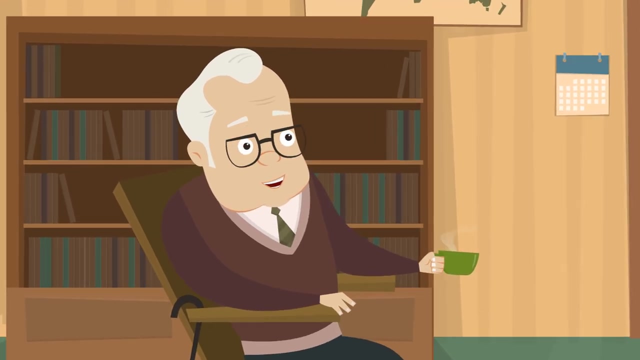 In metropolitan counties, the labor force participation rate is 65% above the national average. However, in counties outside of metropolitan areas, the labor force participation rate is 52%, much lower than the national average. And two as the baby boomer generation ages into retirement.